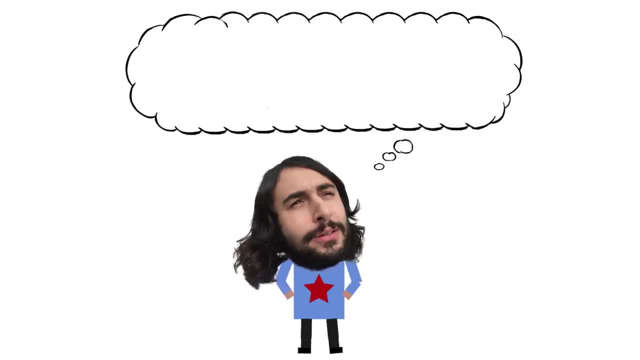 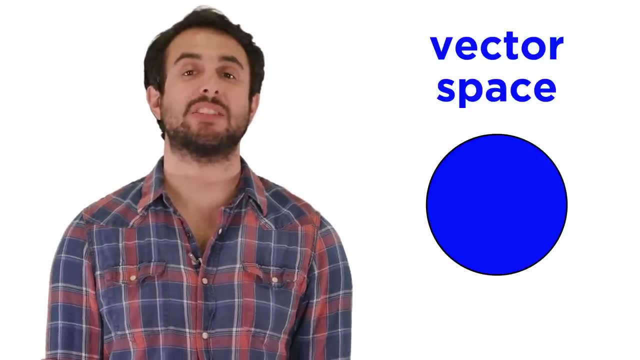 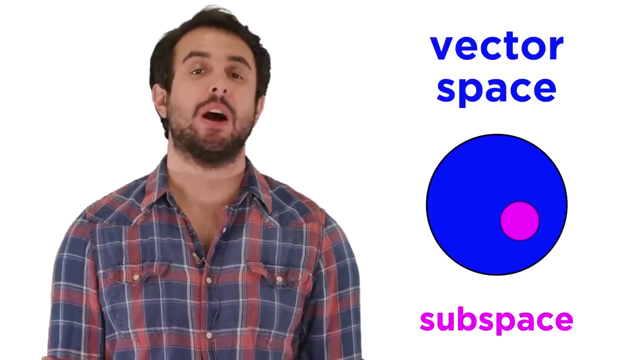 Professor Dave, here let's talk subspaces. Once we understand what makes up a vector space, it is fairly easy to understand the concept of subspaces as well. To put it simply, a subspace is a smaller set within a vector space that is itself a. 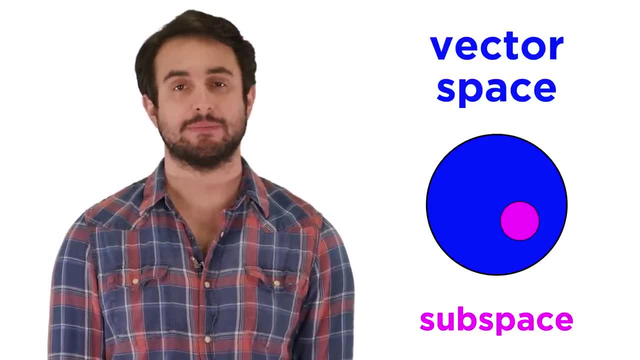 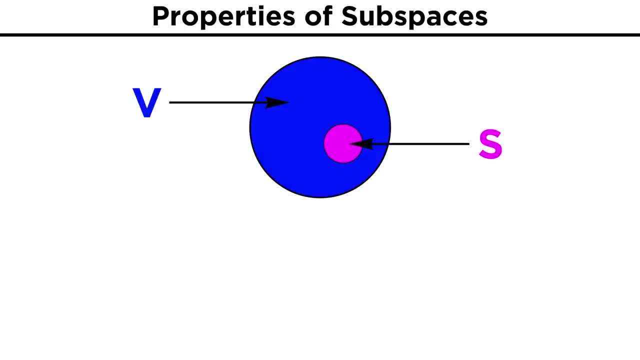 vector space. Let's look at some examples to clarify. Let's say that V is a vector space. Now we can highlight this smaller section of V and call it S. Every element of S was already also in our vector space V, so we know they all obey the properties we discussed. 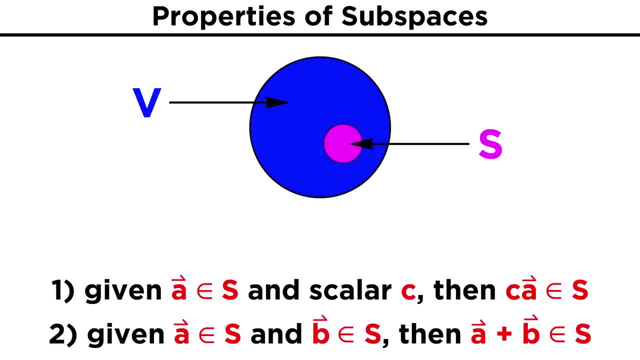 in the previous tutorial. This means that the only requirement we need to check in order to determine whether S is a vector space is that it satisfies the properties of closure. If S is closed, it will also be a vector space and because it is completely contained in. 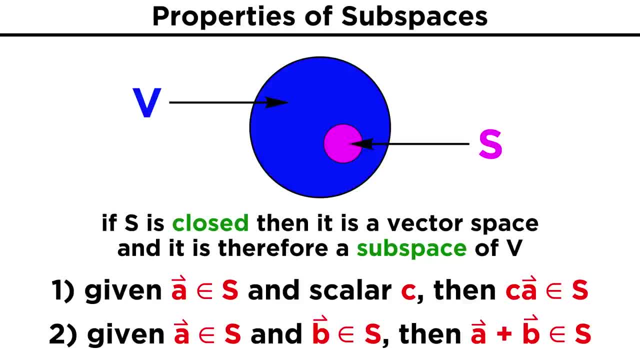 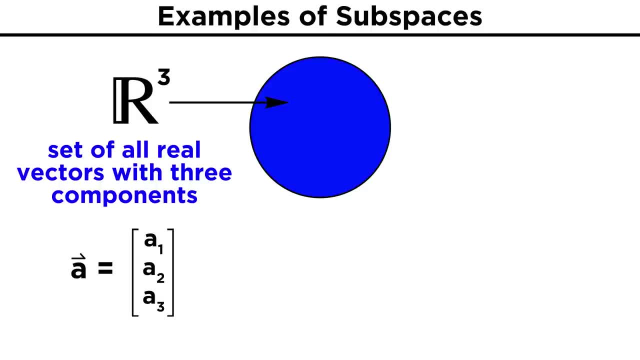 the larger vector space V. we will then call it a subspace of V. We saw last time that R3, or the set of all real vectors of length three, was a vector space. So now let's look at a specific choice of vectors contained within R3 and see if it. 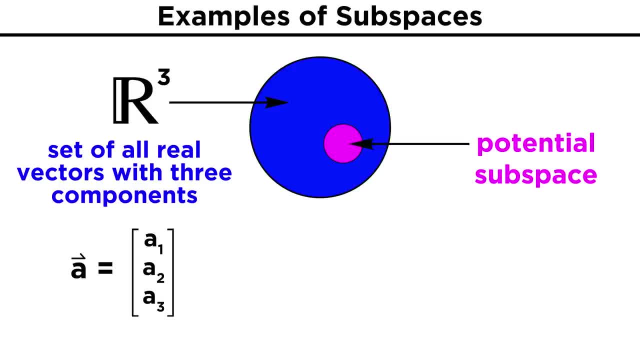 makes up its own vector space. For this example, we will choose a set S made of vectors that have the form By limiting the form of the vector. like this: we have chosen a smaller set of R3, while knowing that our chosen set of vectors still follows the rules of the larger set. 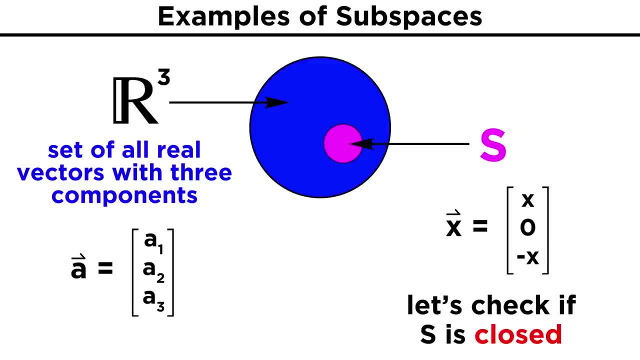 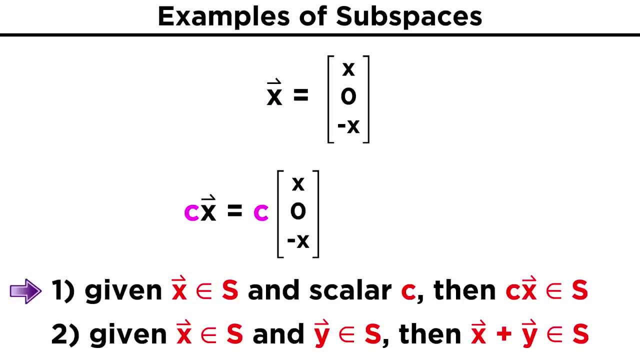 What we must check now is if our smaller set is closed by checking the two properties. First, let's multiply a vector X by a scalar C. Distributing the scalar C, we end up with a vector. Notice that this still has the same form that we want for our set, with some value on the. 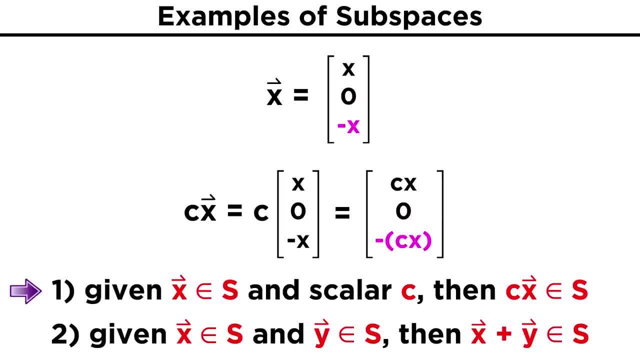 first row, zero for the middle row and the negative version of the first value in the third row. This vector is therefore still in our set S. Next, let's take two vectors, X and Y, both from the set S, and add them together. 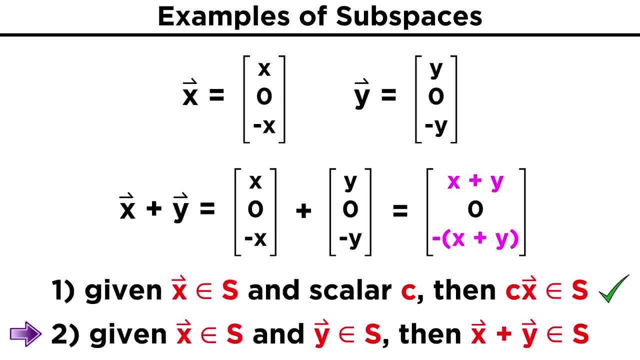 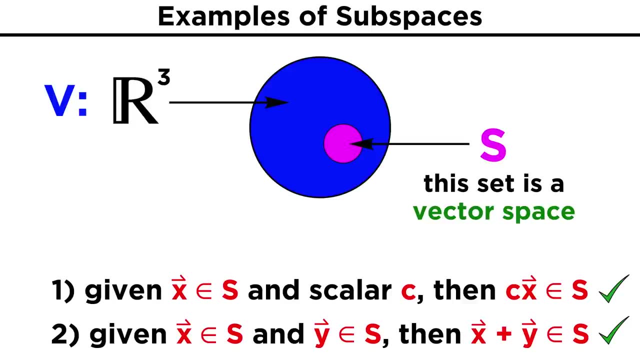 Provided that we factor the negative sign out of this sum, we will see that the third entry is simply the negative version of the first, and once again we find a result in the same form as we started. This means that the sum is also contained in our set S. We have verified that S is closed. 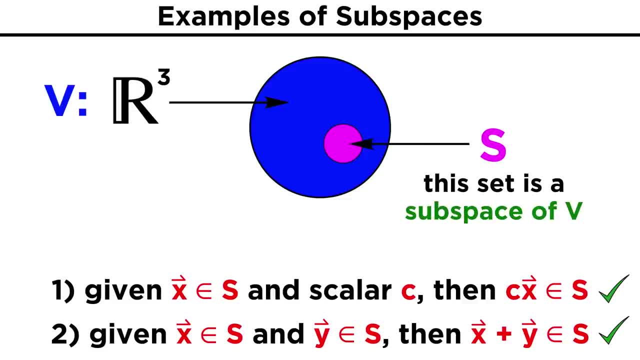 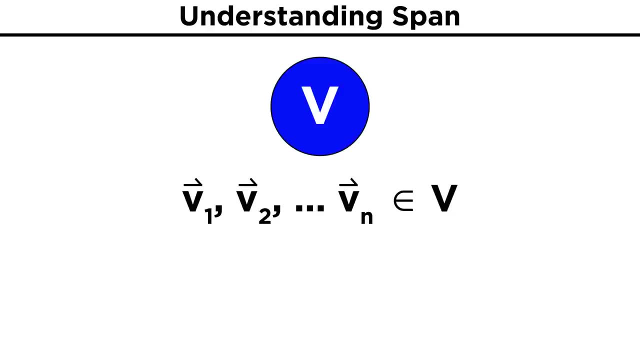 making it a vector space, And because it was contained within the larger vector space, V, this makes S a subspace of V. Before going further, it's important to introduce a few more concepts. Once again, let's say we have a vector space, V, and a number of elements of V which we 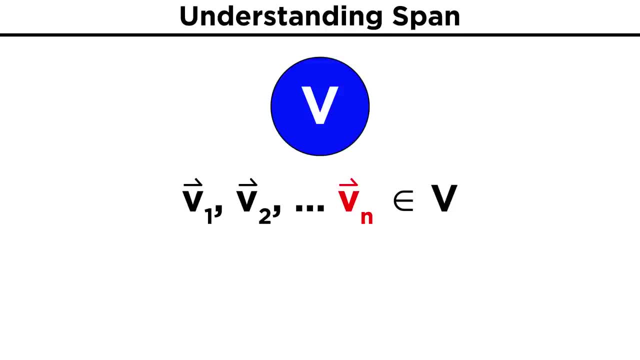 can call V1,, V2, all the way to Vn. Any sum of these elements multiplied by some scalars, which we can represent as, etc. is called a linear combination. The set of all possible linear combinations of these elements is called their span. 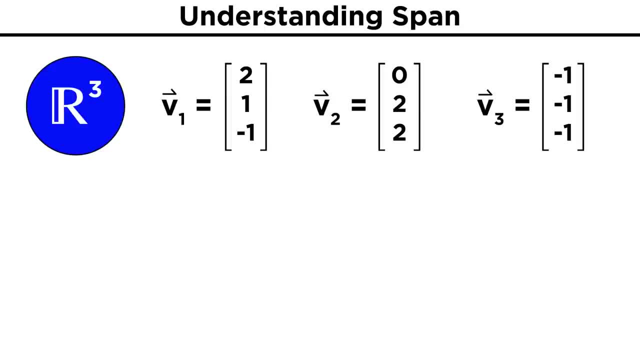 As an example, let's take three vectors from R3, those being two one negative one. zero two, two and negative one. negative one, negative one. The span of these three vectors will be given by the lineal combination. a is constant. 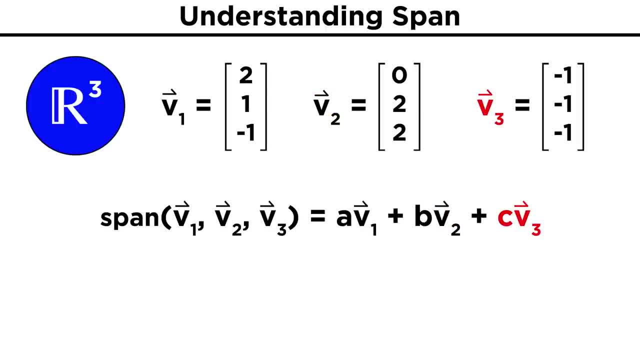 a- v1, plus b- v2, plus c- v3, where a, b and c are all scalars. Let's plug in our vectors and distribute the scalars and then do vector addition to see that the span of these three vectors has the form two a minus c, a plus two, b minus. 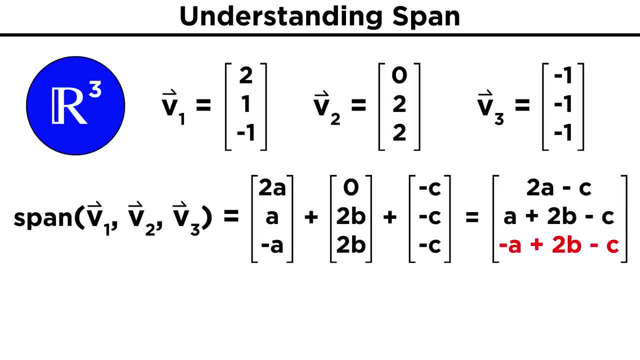 c negative a plus two, b minus c. It's worth noting that the span of any number of elements of a vector space, V, is also a subspace of V. In fact, it is the smallest subspace of V that contains that set of elements.